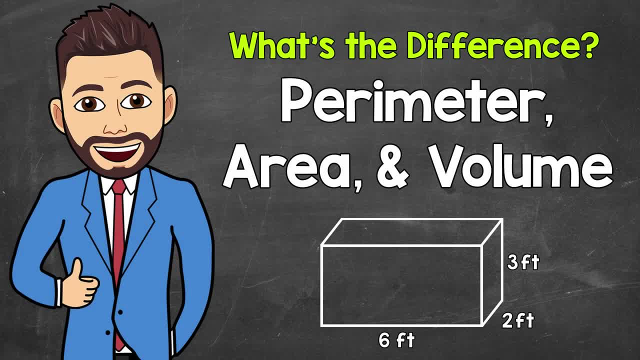 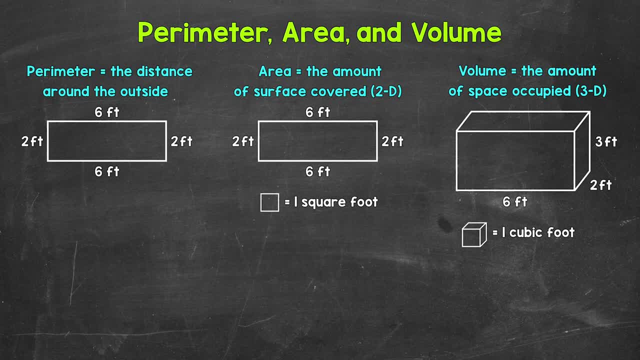 Welcome to Math with Mr J. In this video I'm going to cover what perimeter, area and volume are. We will start with perimeter, move to area and then end with volume. Let's jump into perimeter Now. perimeter is the distance around the outside of a shape. We will use a rectangle for our example of perimeter. 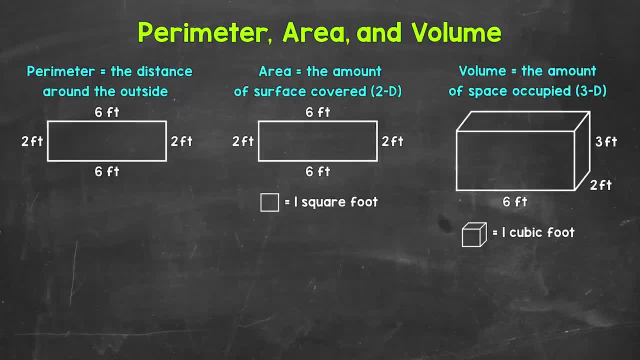 So the perimeter is the distance around the outside of this rectangle. We can find the perimeter by adding the lengths of all of the sides. We have two feet, six feet, two feet and six feet. So perimeter equals two feet plus six feet, plus two feet plus six feet. Now I do want. 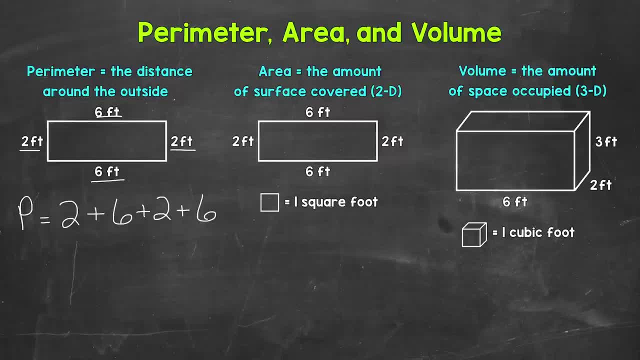 to mention. it does not matter what order you're using. it doesn't matter which order you're using. you add the side lengths in, You get the correct perimeter. however you do it, For example, if we do six plus six plus two plus two, that will give us the same thing and the correct perimeter. So now, 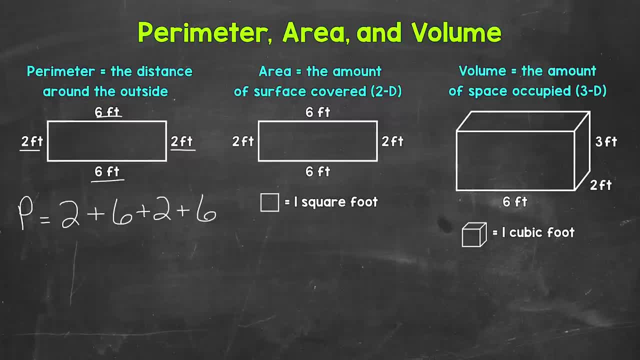 let's add: We have two plus six, that's eight plus two is ten plus six is sixteen. So the perimeter is sixteen feet. So the perimeter of this rectangle, the distance around the outside, is sixteen feet And that's. 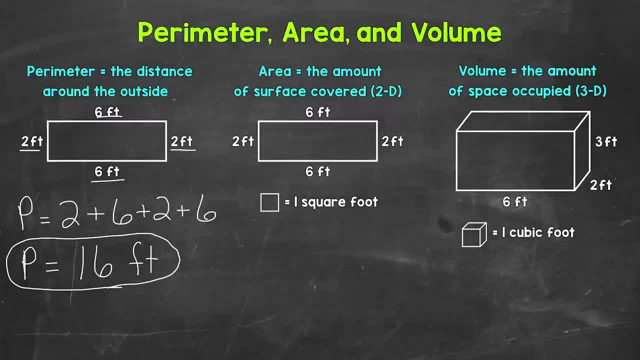 it for perimeter. Just remember: perimeter is the distance around the outside of a shape, a figure, And we can find the perimeter by adding the lengths of all of the sides. Let's move on to area Now. area is the amount of surface a shape covers, and we are talking. 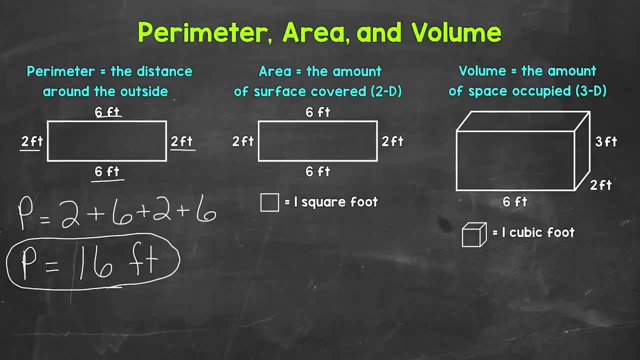 two-dimensional or 2D for area, So the flat surface covered. This is important to keep in mind because once we move on to volume, we will be talking three-dimensional or 3D. So again for area, the amount of surface a shape covers- We measure area in square units. So for our example, 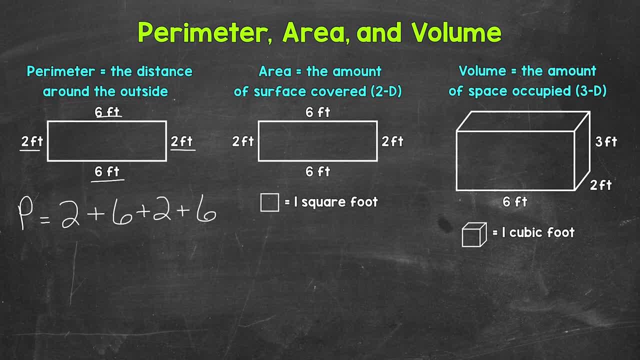 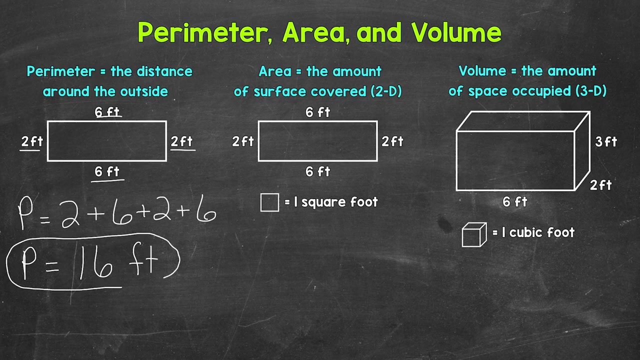 six plus six plus two plus two, that will give us the same thing and the correct perimeter. So now let's add: We have two plus six, that's eight plus two is ten plus six is sixteen, So the perimeter is sixteen feet. So the perimeter of this rectangle, the distance around the outside, is: 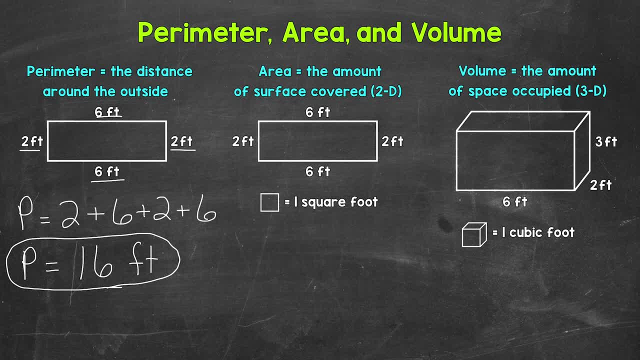 sixteen feet. and that's it for perimeter. Just remember, perimeter is the distance around the outside of a shape, a figure, and we can find the perimeter by adding the lengths of all of the sides. Let's move on to area Now. area is the amount of surface a shape covers. 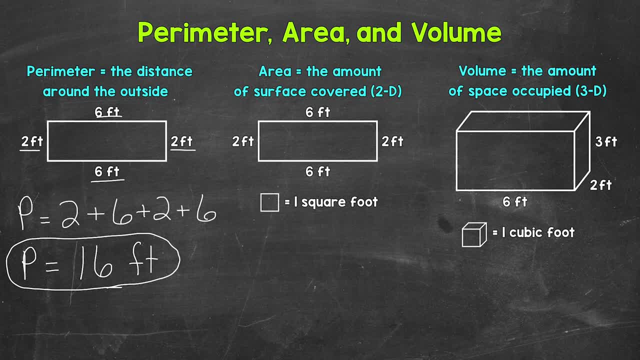 and we are talking two-dimensional or 2D for area, so the flat surface covered. This is important to keep in mind because once we move on to volume, we will be talking three-dimensional or 3D. so again for area, the amount of surface a shape covers. We measure area in square units. 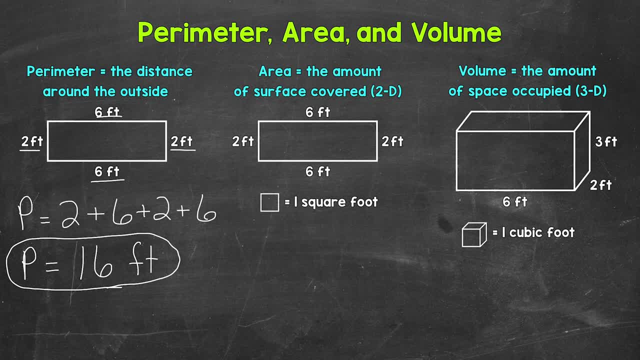 so, for our example, we have a rectangle and we are working with feet for our unit of measure. So what we need to do, we need to see how many square feet this rectangle covers. This is a square foot right here, so it is one foot by one foot. So again, we're going to see how many square 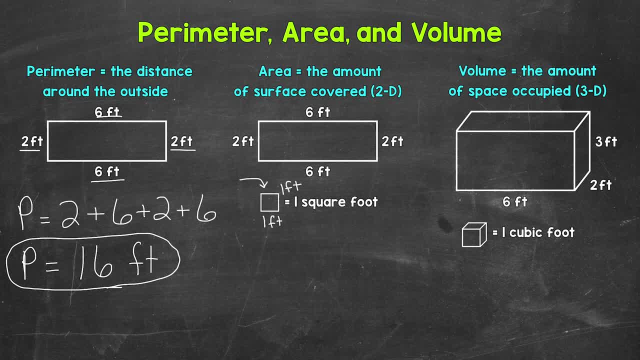 feet that this rectangle covers. Let's see what this looks like. So let's start with this. six feet right here. so for the length of six feet, we have six feet going across. so let's draw out the six feet. So one, two, three, four, five and six. 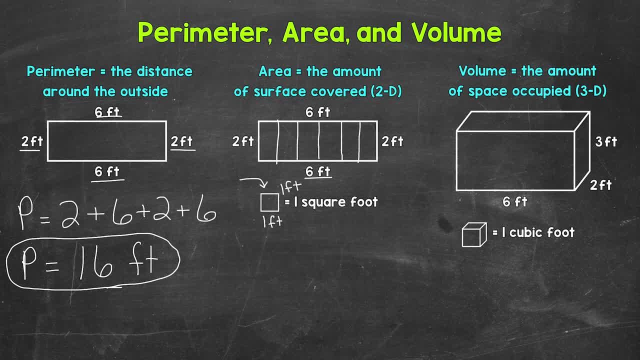 Now for our width, which we are going the other way. we have two feet, So let's draw out two feet, One, two going that way distance over' 5 metres per inch. Seriously, what the heck was that for? 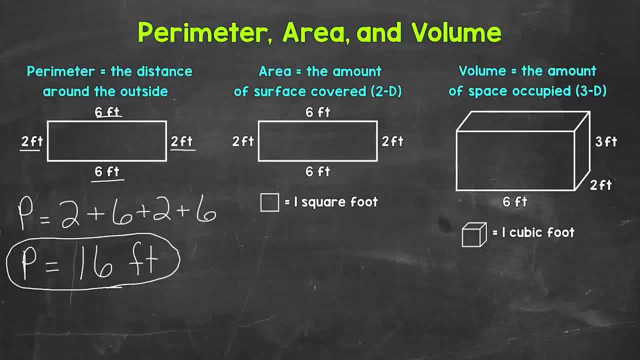 we have a rectangle and we are working with feet for our unit of measure. So what we need to do, we need to see how many square feet this rectangle covers. This is a square foot right here, So it is one foot by one foot. So, again, we're going to see how many. 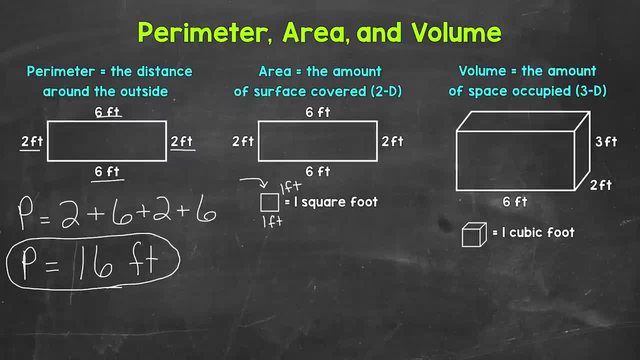 square feet that this rectangle covers. Let's see what this looks like. Let's start with this: six feet right here, So the length of six feet. We have six feet going across. Let's draw out the six feet, So one, two, three, four, five and six. Now for our width. 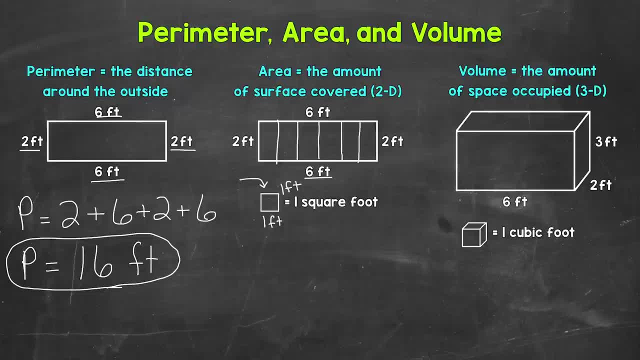 which is going the other way. we have two feet, So let's draw out the two feet, So one, two feet going that way. Now we have the square feet that this rectangle covers. So how many square feet does it cover? Let's draw out the six feet, So one, two, three, four, five and six. Now we have. 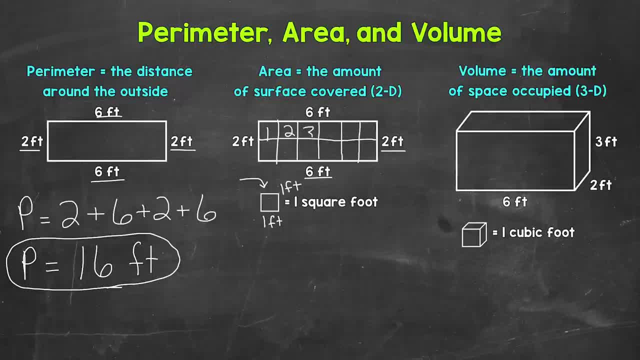 Well, one, two, three, four, five, six, seven, eight, nine, ten, eleven, twelve. So the area of this rectangle is twelve square feet. Now for area. we put that two. there We have our unit of measure, feet. 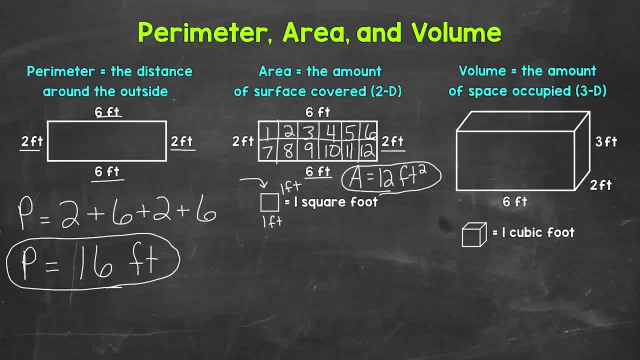 to the power of two To represent square feet. the exponent only applies to the unit of measure, by the way, not the number, So don't get confused by that. Again, that just represents square feet, or whatever your unit of measure is. Now for this example, we drew out all of the square feet to 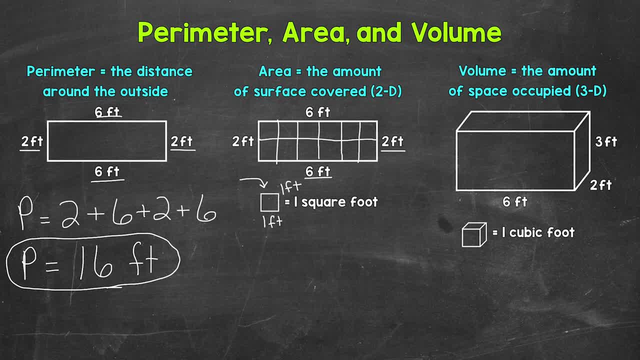 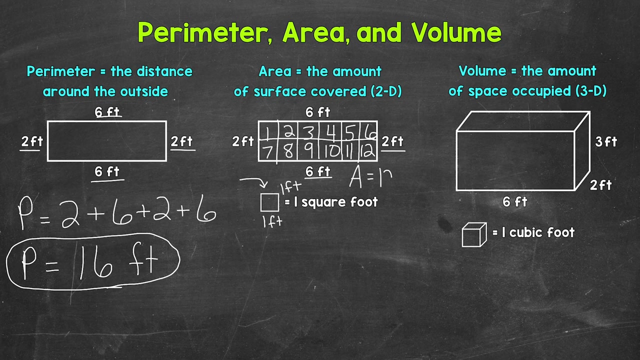 getting. So let's start with this. six feet here, 6ˆ the length. we have six feet going across. we have the square feet that this rectangle covers. So how many square feet does it cover? Well, 1,, 2,, 3,, 4,, 5,, 6,, 7,, 8,, 9,, 10,, 11, 12.. So the area of this rectangle is 12 square. 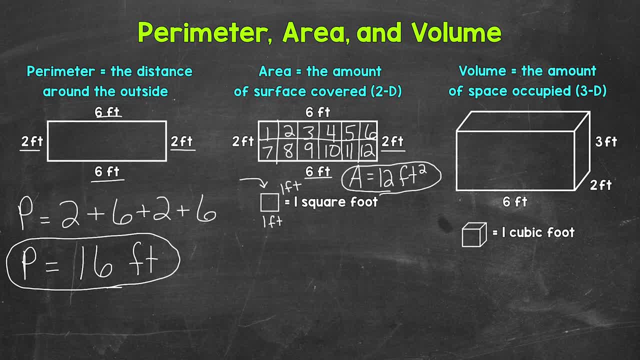 feet. Now for area. we put that 2. there We have our unit of measure: feet to the power of 2, to represent square feet. The exponent only applies to the unit of measure by the way, not the number, So don't get confused by that. Again, that just represents square feet. 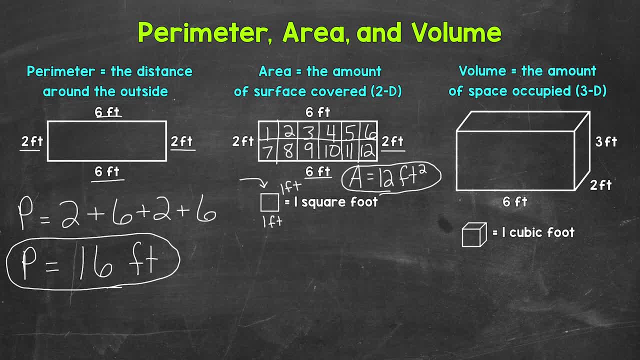 or whatever your unit of measure is. Now for this example, we drew out all of the square feet to show what we have. So we have a square feet and we have a square feet, and we have a square- What area looks like and how it is measured. For a rectangle, we can just use the formula. 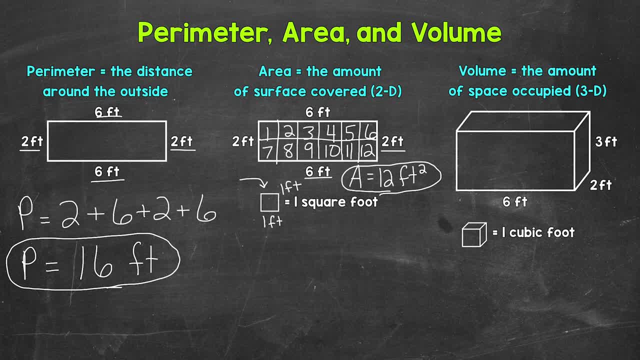 area equals length times width. So area equals length times width. And I used a cursive L so it doesn't look like a 1.. Now we can plug in the length and the width, So area equals, and we're going to use 6 feet for the length. 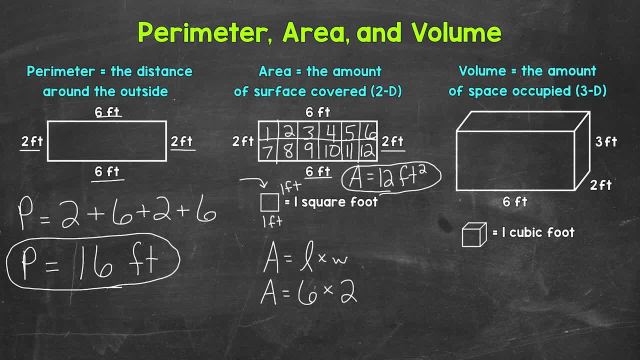 times 2 feet for the width. Now I used the longer side, 6 feet for the length, But if you were to switch those, you'll still get the correct area. Now we can multiply. So 6 times 2 gives us an area. 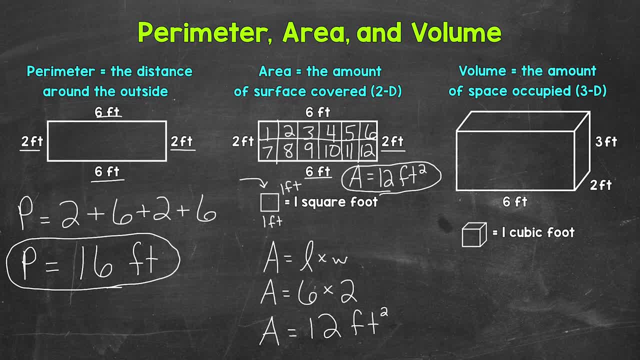 of 12 square feet. So you can see that we get 12 square feet that way as well. And remember, we use that 2 for the length and we get the correct area. So 6 times 2 gives us an area of 12 square feet. 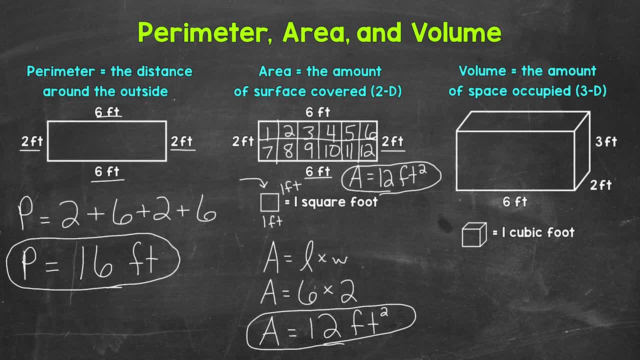 2 for area, to show that we measure area in square units And for this example it was square feet. This rectangle covers 12 square feet And that's it for area. Just remember, area is the amount of surface something covers. Now something to keep in mind. we find area of different shapes. 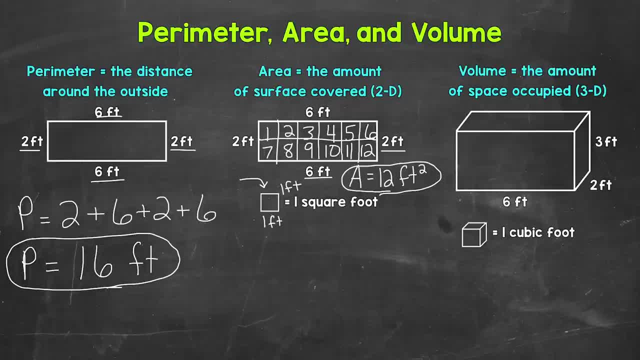 show what area looks like and how it is measured. For a rectangle we can just use the formula: area equals length Times width. So area equals length times width, And I used a cursive, L, so it doesn't look like a one. Now we can plug in the length and the width, So area equals, and we're going to use 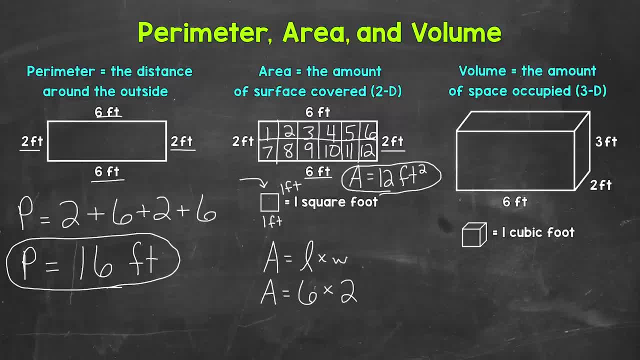 six feet for the length times two feet for the width. Now I used the longer side, six feet for the length. But if you were to switch those, you'll still get the correct area. So area equals length times width. Now we can multiply. So six times two gives us an area of 12 square feet. 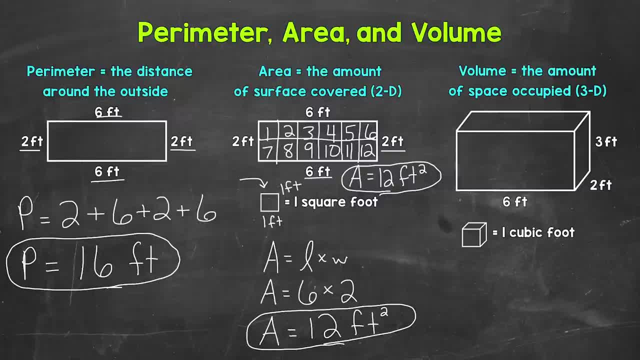 So you can see that we get 12 square feet that way as well, And remember we use that two for area to show that we measure area in square units And for this example it was square feet. This rectangle covers 12 square feet, So we can see that we get 12 square feet, And remember we use 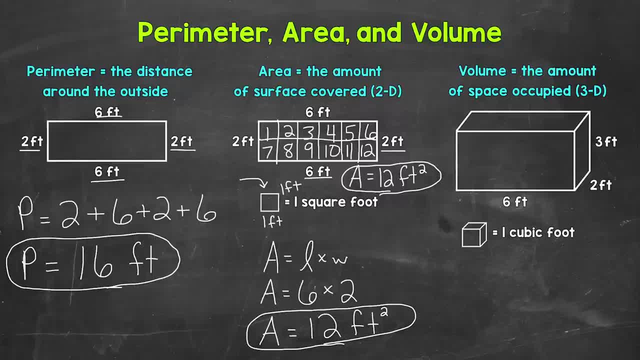 And that's it for area. Just remember, area is the amount of surface something covers. Now something to keep in mind. we find area of different shapes and figures, different ways. There are different formulas. We used length times width because we had a rectangle, for our example. Let's move on to 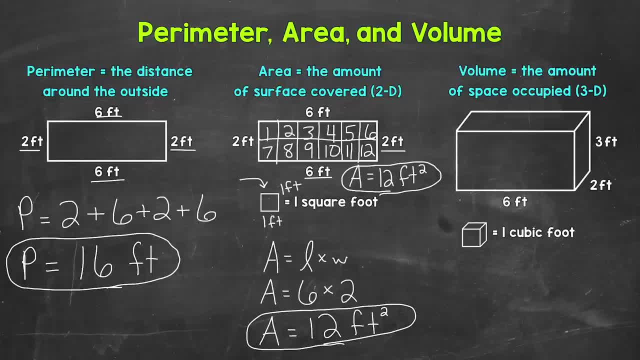 volume. Now, volume is the amount of space occupied by a three-dimensional, a 3D, shape. So we are moving from area which is two-dimensional or flat, and we are moving to volume which is three-dimensional, 3D. So instead of square units, like we used for area, we measure. 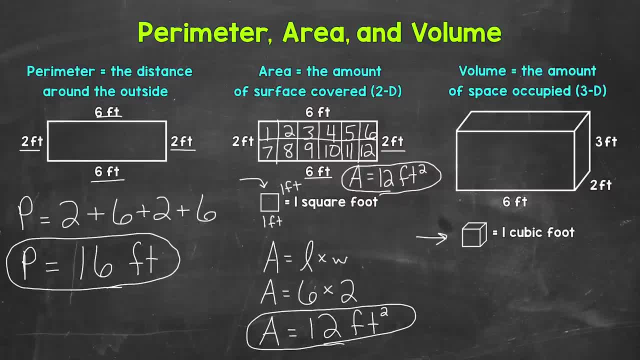 volume in cubic units. For our example, we have a rectangular prism and we are working with feet again for our unit of measure. What we need to do, we need to see how many cubic feet this rectangular prism occupies or takes up. A cubic foot is a one foot by one foot by one foot cube. 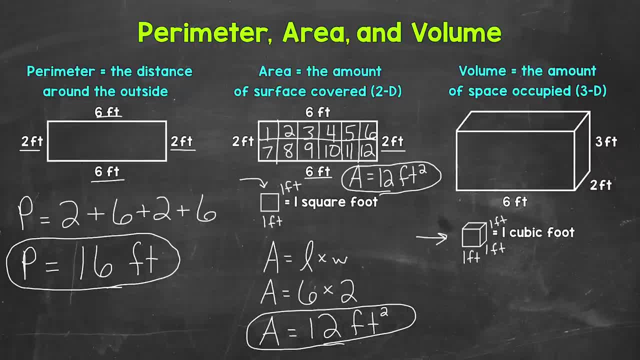 Let's see what this looks like. We have six feet for our length, So let's draw out six feet here. So one, two, three, four, five and six, The six feet. The six feet go across the top as well. And then we have two feet for the width, So let's draw two. 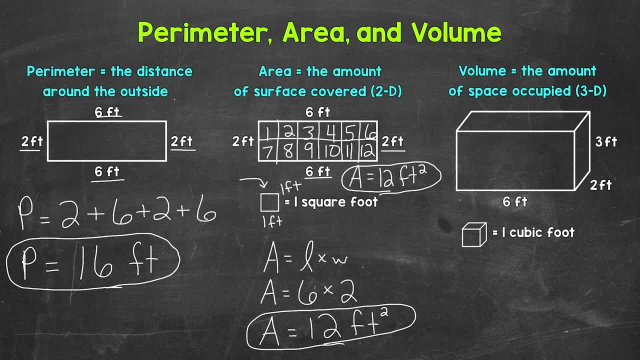 and figures different ways. There are different formulas. We used length times width because we had a rectangle, for our example. Let's move on to volume Now. volume is the amount of space occupied by a three-dimensional, a 3D shape. So we are moving from area which is two-dimensional or flat. 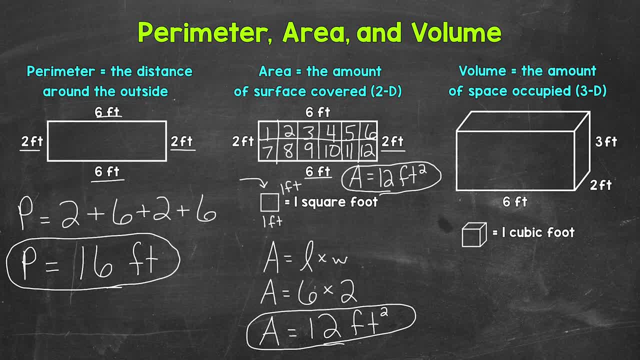 and we are moving to volume, which is three-dimensional, 3D. So instead of square units, like we used for area, we measure volume in cubic units. For our example, we have a rectangular prism And we are working with feet again for our unit of measure. 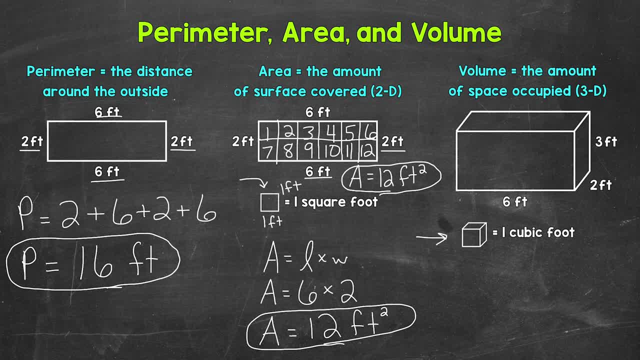 What we need to do. we need to see how many cubic feet this rectangular prism occupies or takes up. A cubic foot is a 1 foot by 1 foot by 1 foot cube. Let's see what this looks like. We have six feet for our length, So let's draw out six feet here. 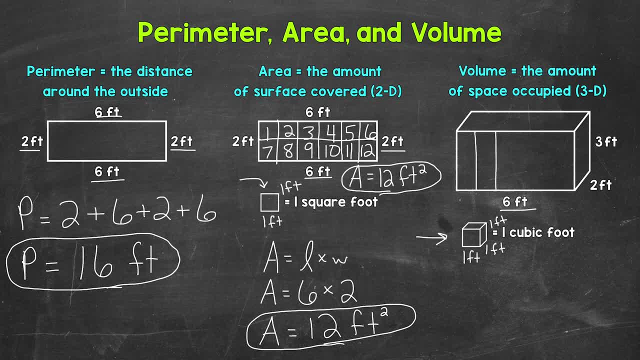 So 1,, 2,, 3,, 4,, 5, and 6.. The 6 feet go across the top as well, And then we have 2 feet for the width. So let's draw 2 feet here. 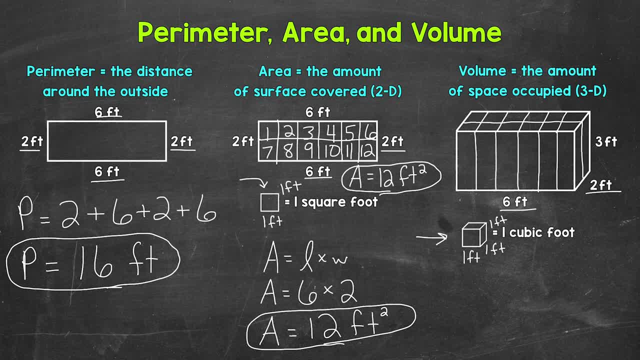 And then this goes across the top as well, And then we have a height of 3 feet, So 1,, 2, and 3.. Now we have the amount of cubic feet that this rectangular prism occupies. Now, since this is 3D, we can't see all of the cubes. 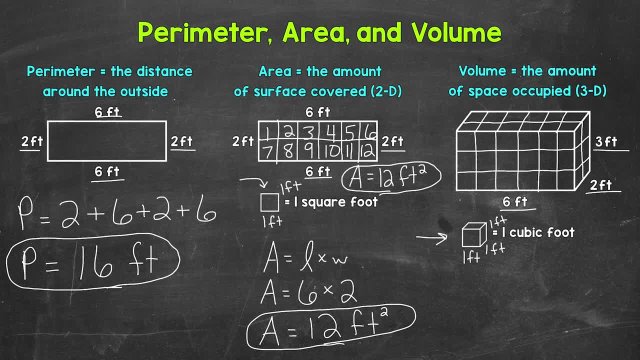 Not all of them are visible, But we can still figure out how many cubes there are. In order to do this, let's take a look at the bottom layer. We have 6 cubes going across and 2 cubes going back, So 6 by 2.. 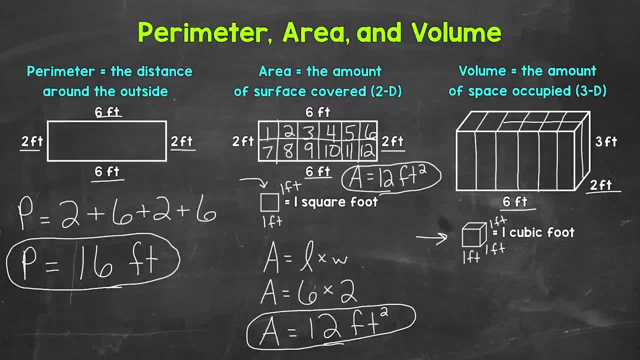 feet here, And then this goes across the top as well, And then we have a height of three feet. So one, two and three. Now we have the amount of space occupied by a three-dimensional, a 3D shape. So let's draw two feet here, And then this goes across the top as well, And then we have a height of three feet. So one, two and three. Now we have the amount of space occupied by a three-dimensional, a 3D shape. So let's draw two feet here, And then this goes across the top as well, And then we have a height of three feet. So one, two and three. 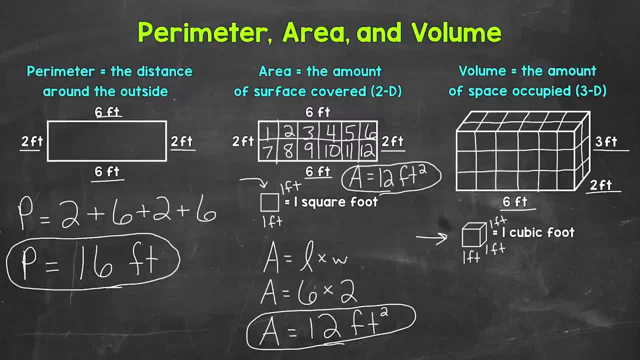 Now we have the amount of cubic feet that this rectangular prism occupies. Now, since this is 3D, we can't see all of the cubes- Not all of them are visible, but we can still figure out how many cubes there are. In order to do this, let's take a look at the bottom layer. 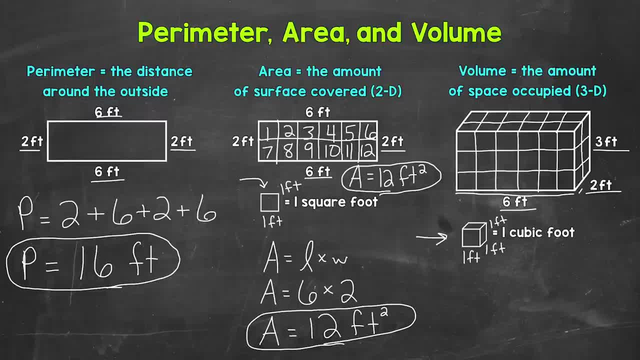 We have six cubes going across and two cubes going back. so six by two That gives us 12 cubes on the bottom layer. And then we have three layers: one, two, three. So we have 12 cubes on this layer, 12 cubes on this layer and 12 cubes on this layer. 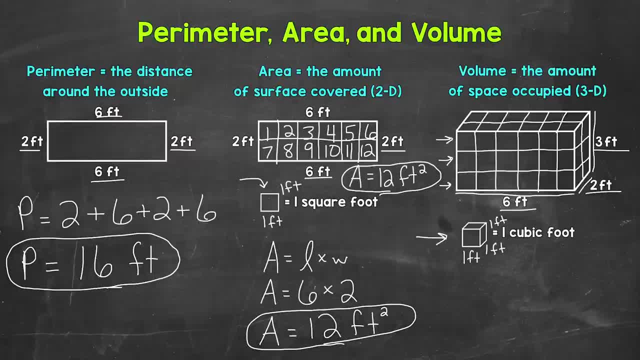 So 12,, 12, and 12, or 12 times 3.. That gives us 36 cubic feet, So the volume equals 36.. Now for volume. we use that 3,, so our unit of measure feet is to the power of 3 to represent cubic feet. 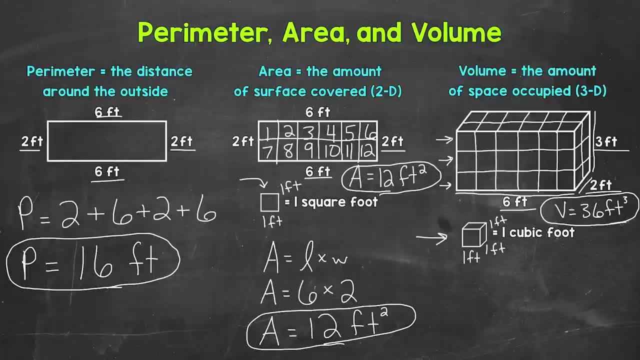 We measure volume in cubic units. Now we drew out all of those cubes to show how we measure volume For a rectangular prism. we can just use volume equals length. We can also use length times width times height And we can plug in the length, width and height. 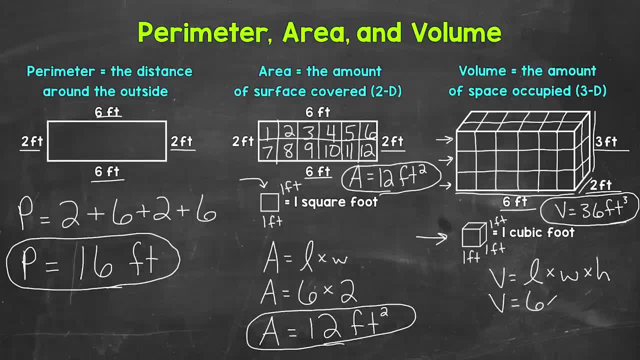 So the length we are going to use 6 feet, times the width of 2 feet, times the height of 3 feet, And then we can multiply: 6 times 2 is 12, times 3 is 36..